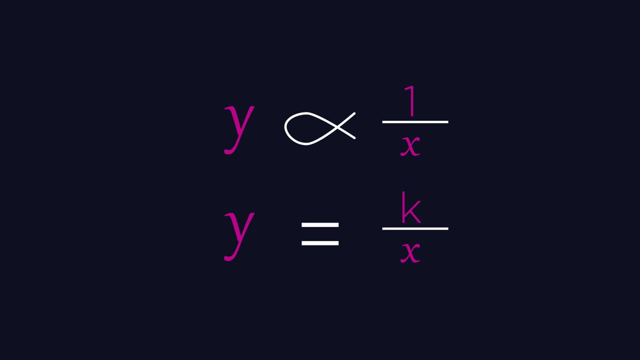 k is the constant of proportionality which, for inverse proportion, is the product of two quantities. You may be asked to give a formula for the relationship between two quantities or to find a value. Consider this question If you want to have a go yourself. 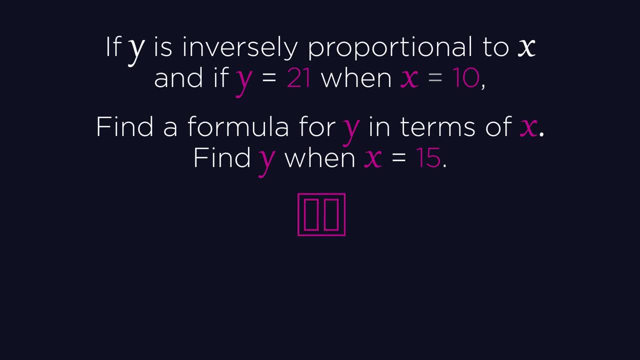 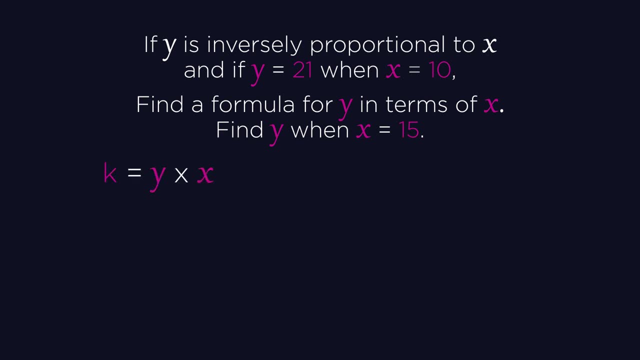 pause the video now To find the formula for Y in terms of X, when you first need to find k, the constant of proportionality, Because for inverse proportion k is the product of the quantities x and y. we multiply these. 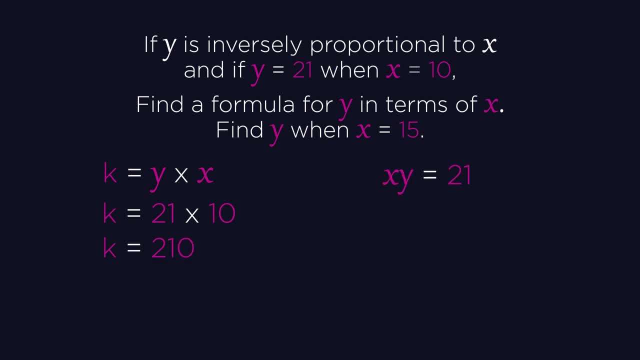 k is a value of 210, so xy equals 210.. To put this equation in terms of Y, we rearrange dividing through X to give us an answer of y equals 210 over x. To find the value of y when x equals 15, we can substitute the value for x into the equation. 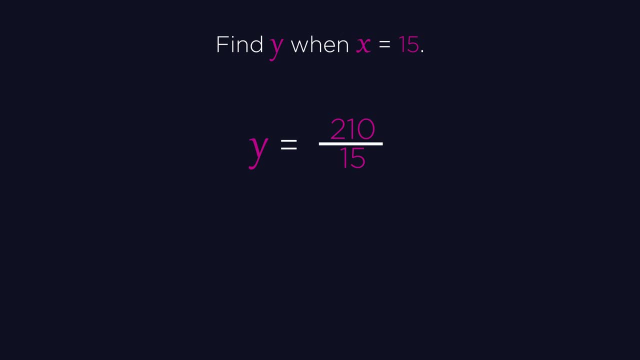 meaning y is equal to 210 divided by 15.. This means the value for y is 14.. You may also encounter inverse proportion questions involving indices. For example, y is inversely proportional to the square of x. y equals 20 when x equals 3.. 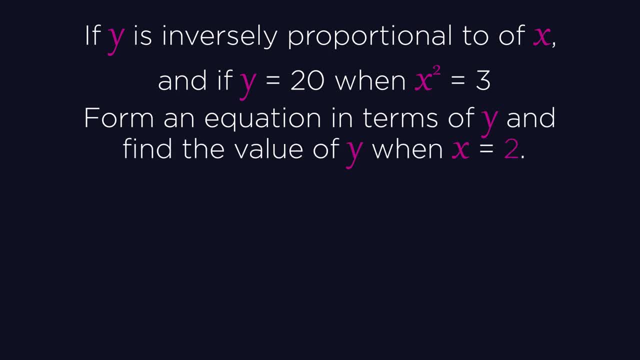 Form an equation in terms of y and find the value of y when x equals 2.. If you would like to have a go at this, pause the video now, Because in this question the proportional quantities are y and x squared. the constant k links these values, not y and x. 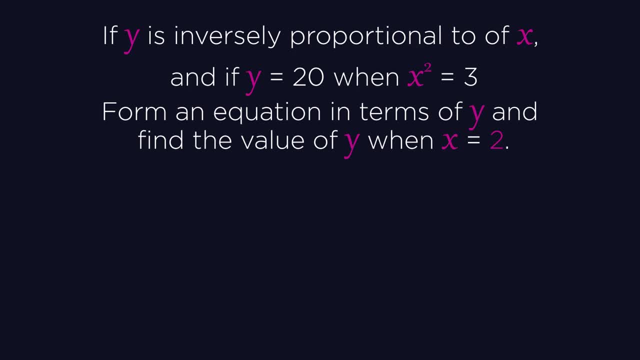 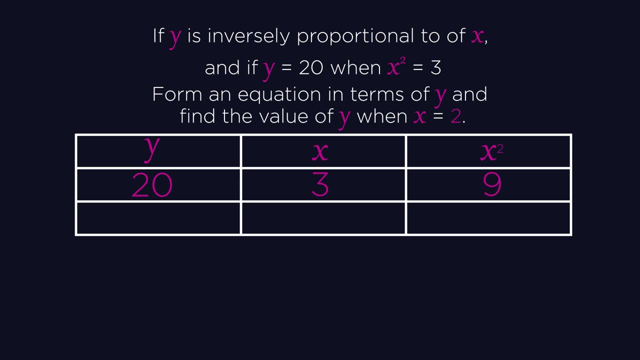 We therefore need to know the x squared values. You can use a table like this to help lay out the values. k is again the product of x squared and y, So x squared equals y equals 180.. So y equals 180 over x squared in terms of y. 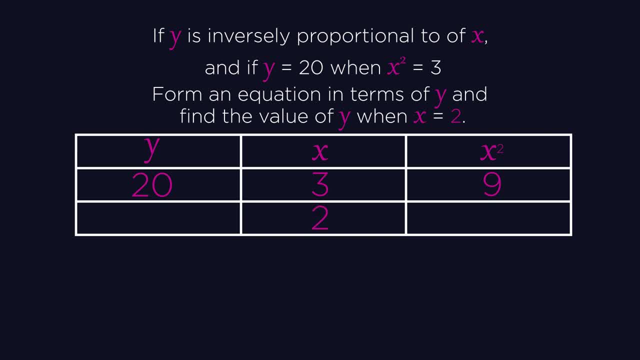 Try and see if you can now find the value of y when x is 2.. Pause and have a go. When x is 2, x squared is 4.. If we substitute this into our equation, x squared equals 180 over x squared.